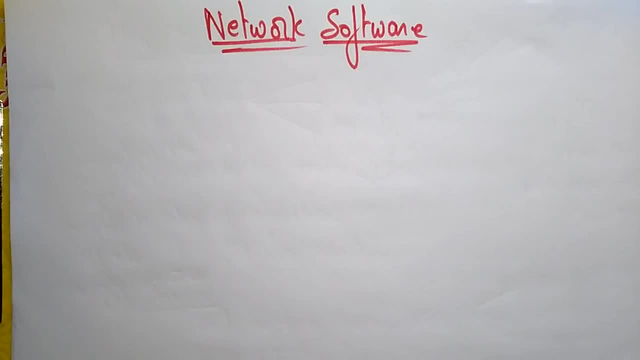 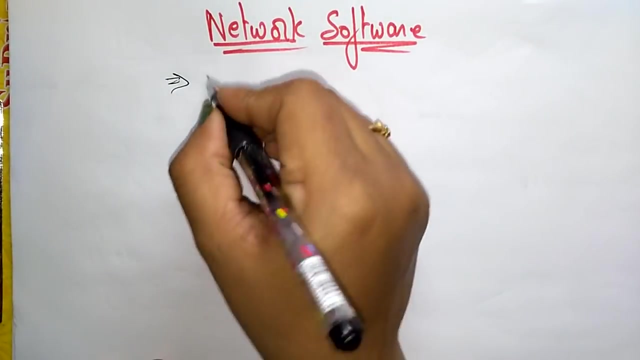 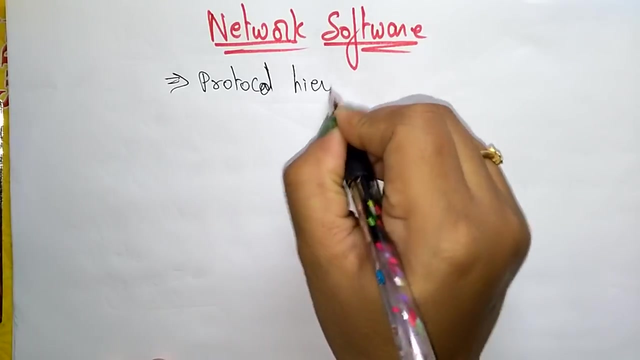 Hi students, coming to the next topic in computer networks, that is the network software. So for every networking there is a software and for that software there is some set of rules and protocols that we have to follow. So the network software is also having some, some design issues, like they can be. choose first the protocol hierarchy. The network software first has to see the protocol hierarchies, that is the layered structure. 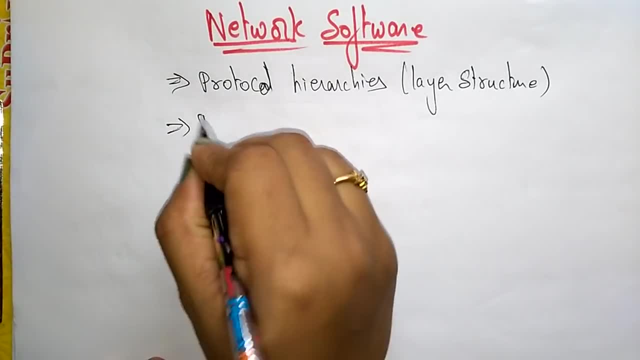 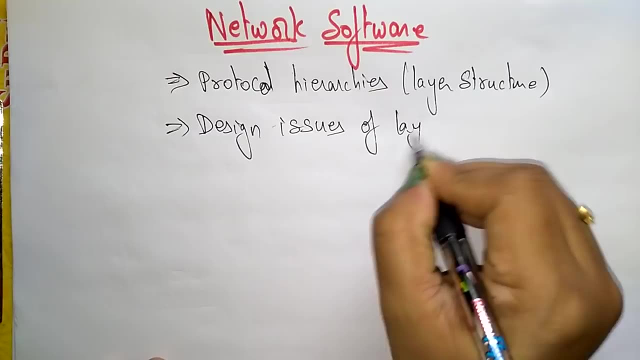 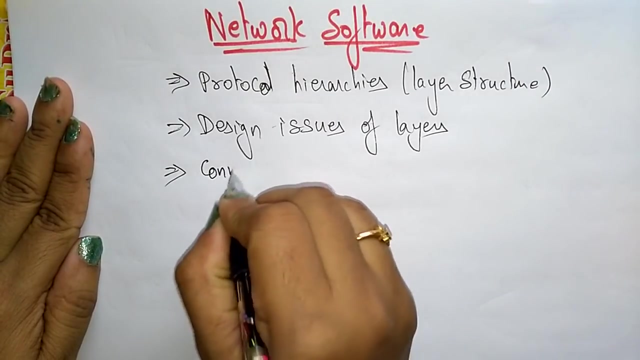 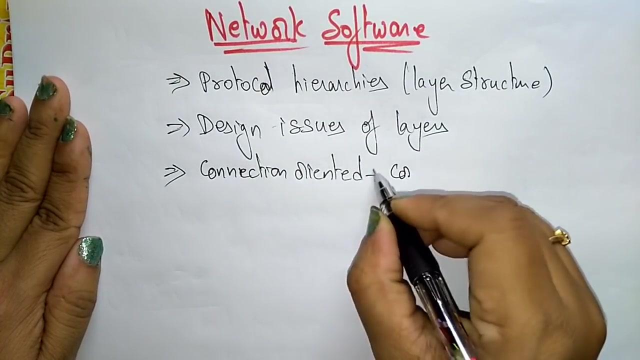 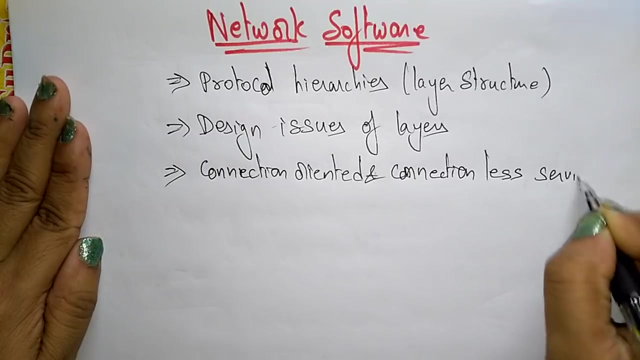 Next it has to, it has to think about the design issues of layers, Design issues of layers. and next it has to think the network software has to check whether it is a connection oriented between the layers, connection oriented or connection less, connection less service between the layers. and this network software is also having some set of rules and protocols that we have to follow. 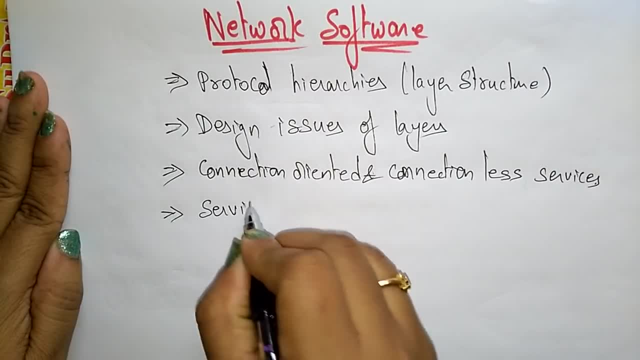 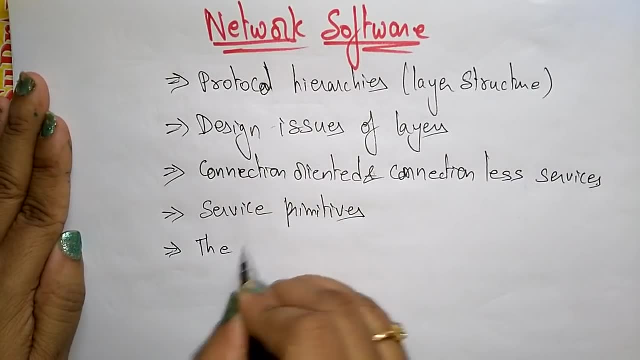 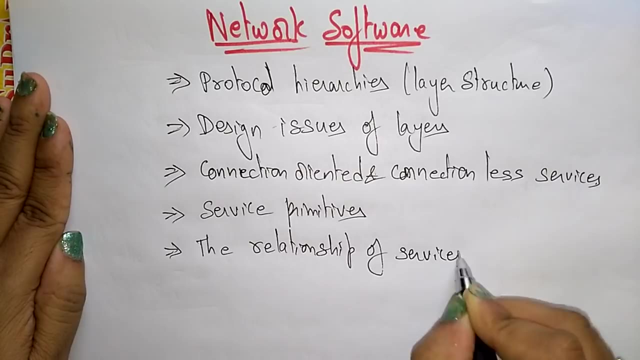 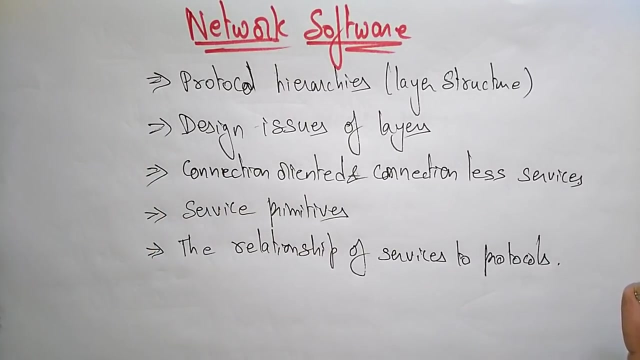 So it has to check the service primitives between the layers. What are the service primitives that are present? service operations between the layers, and it studies the relationship between relationship of services to protocols. So these are the issues that the network software will think in the network layer. So, whatever the network we are thinking about that. 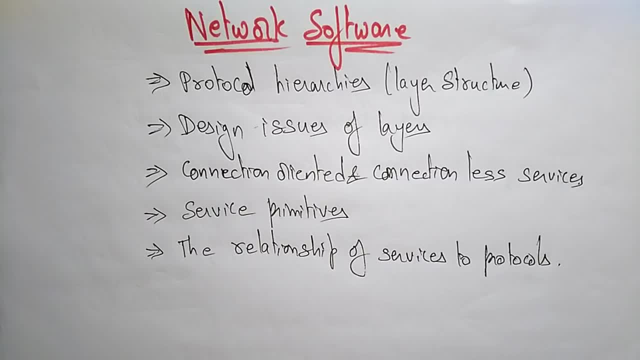 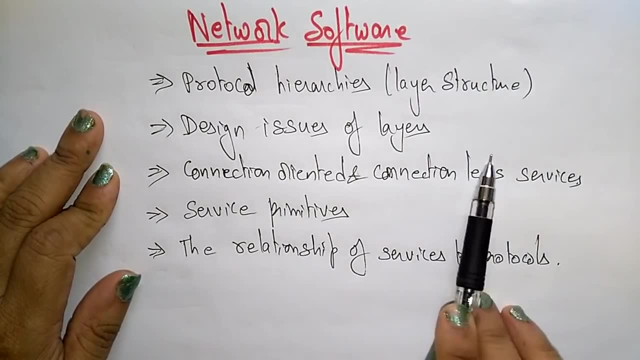 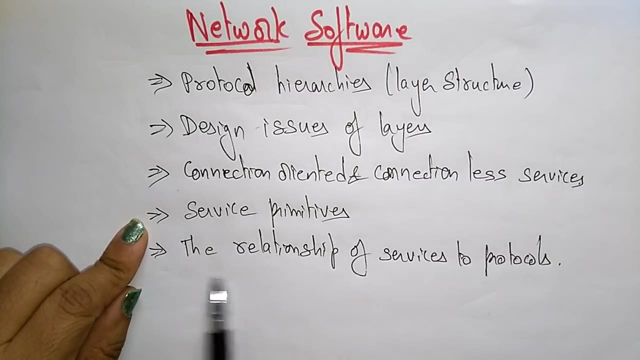 We are using from host one host to another host. So the software that we are using that has to check whether the the protocol hierarchy that is a layered structure and it sees the design issues of each layers and the connection oriented or connection less services are providing is a service, service primitives and the relationships of service of protocols. 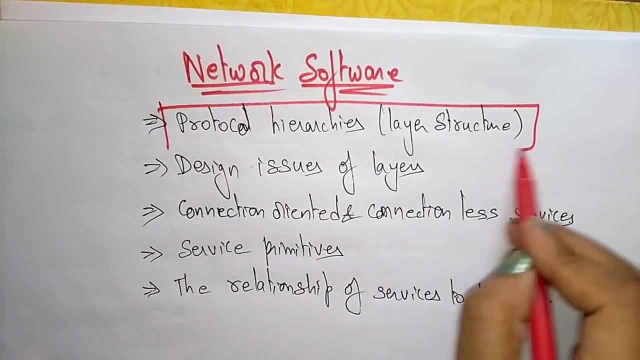 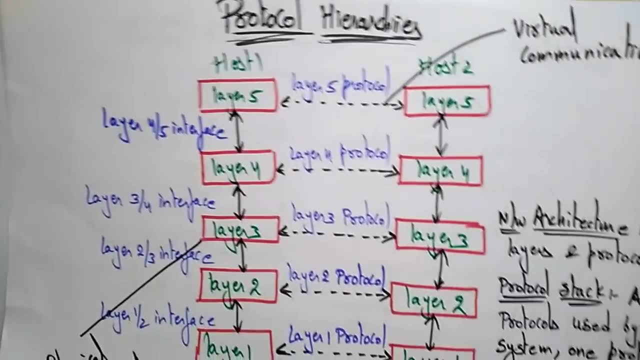 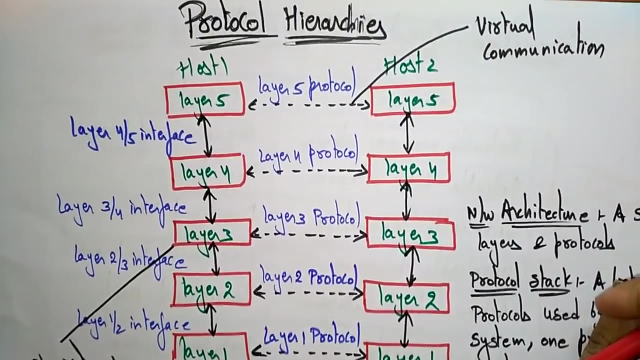 Now let us see what is this protocol hierarchy first. Now let us discuss about the protocol hierarchy in the network software. So this is a protocol hierarchy. So this protocol hierarchy is total, having the four, five layers total one, two, three, four, five. total it is having the five layers. 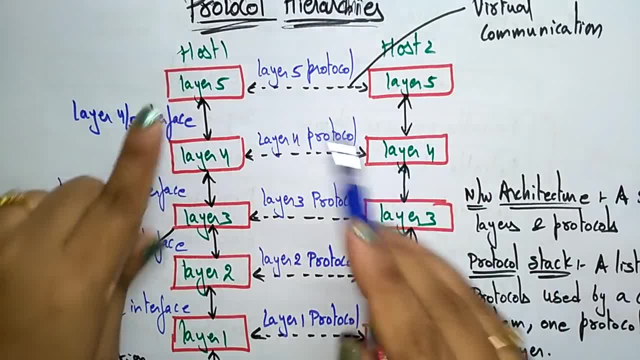 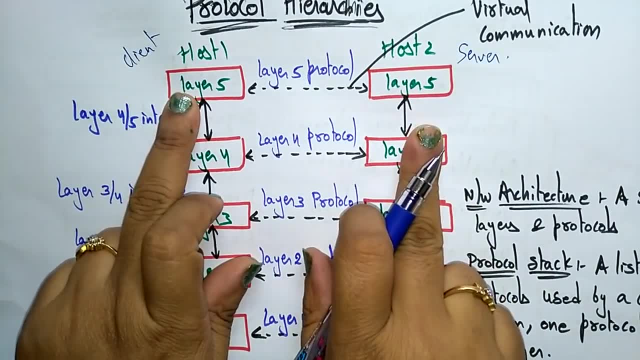 So one is a host one and host two. So this host one is just: you can take it as a client, or you can take the server Two computers, or you can take the two computers, or you can take this is a client and this is a server, or both servers or both clients. 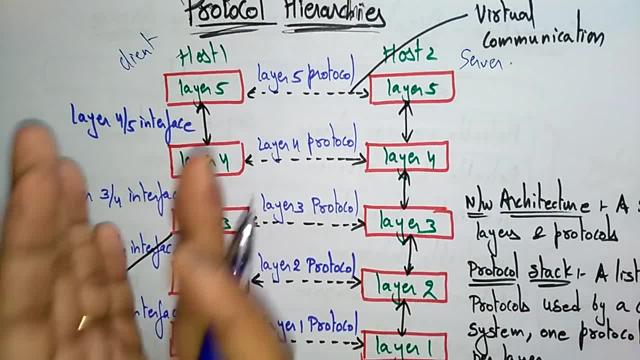 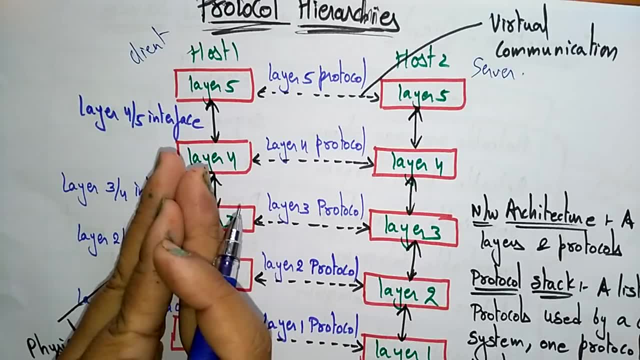 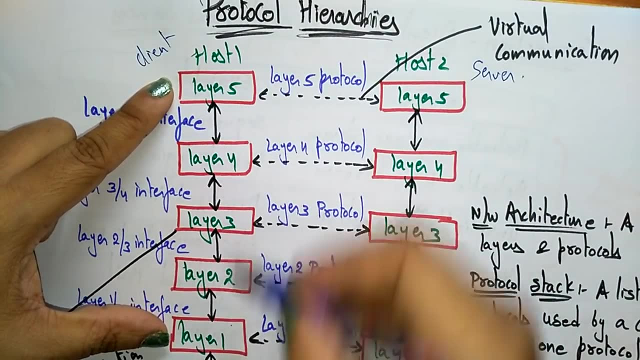 Whatever it may be OK. So just imagine these are the two computers. This is one computer and this is another computer. So in the network, these computer, whatever the computer host one we are using client, one client. they are divided into five layers: Layer five, layer four, layer three, layer two, layer one. 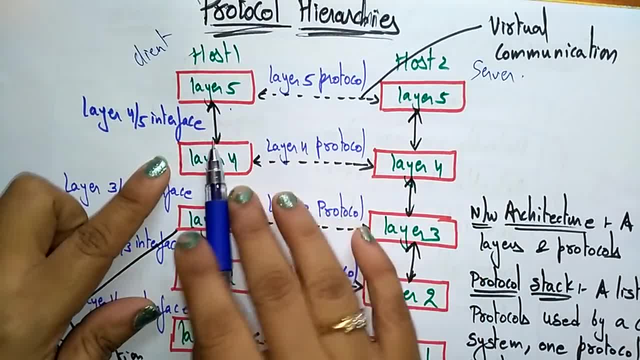 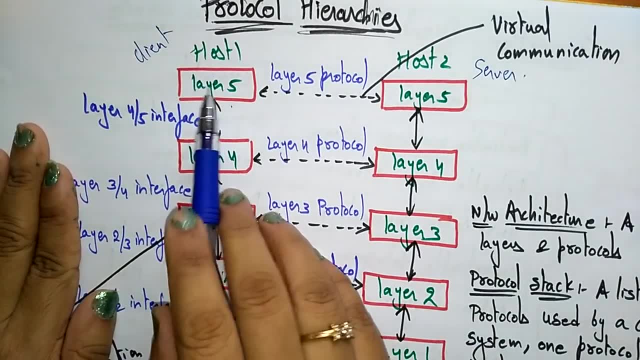 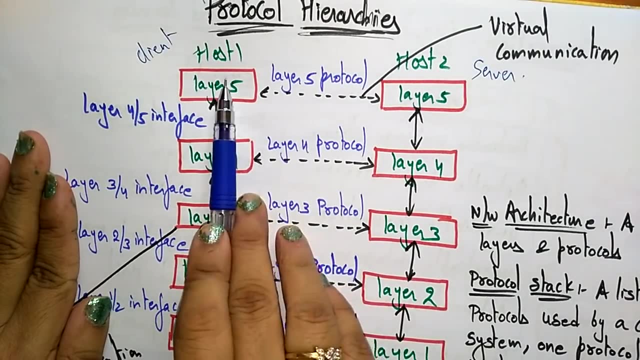 So layer five is just an application layer. So everything that we will discuss later. But just I'm explaining about the protocol hierarchy Here. So this layer, host one, is communicated with the host two with layer protocols, a protocol connections will be there between one computer to another company computer. 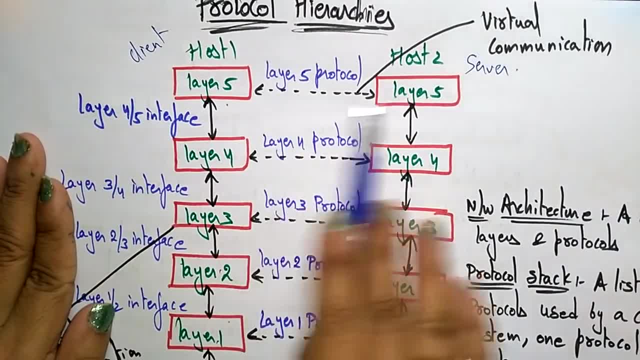 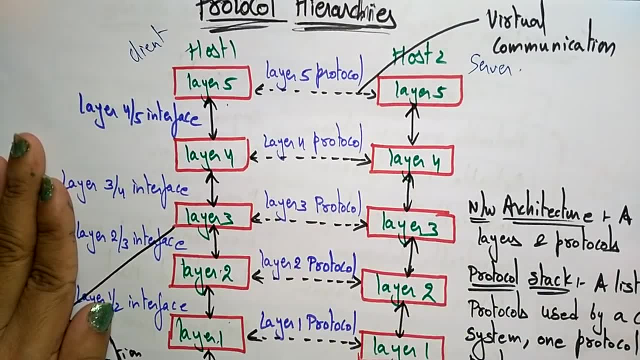 So this protocol is nothing but a virtual communication. This is not the physical thing, So it's just a virtual signal from host one to host two that you call it as a protocol. A protocol is nothing, but it is a rule, set of rule which is forming a virtual communication. 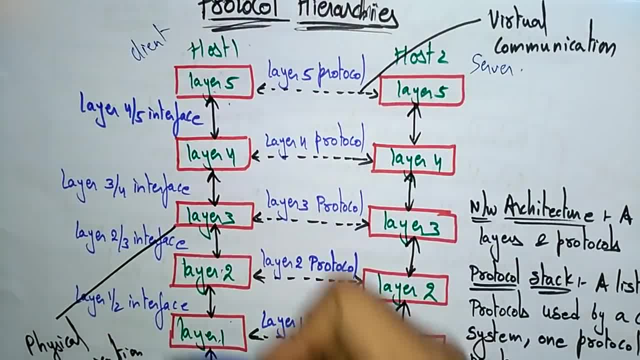 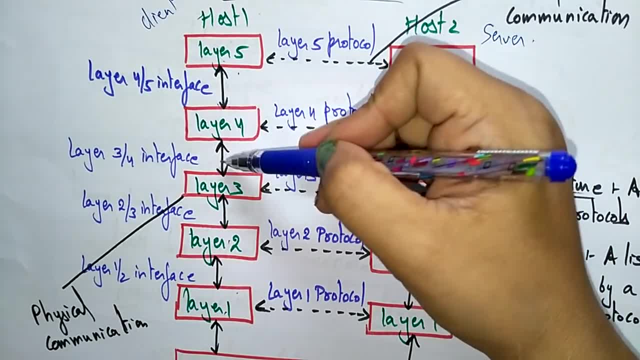 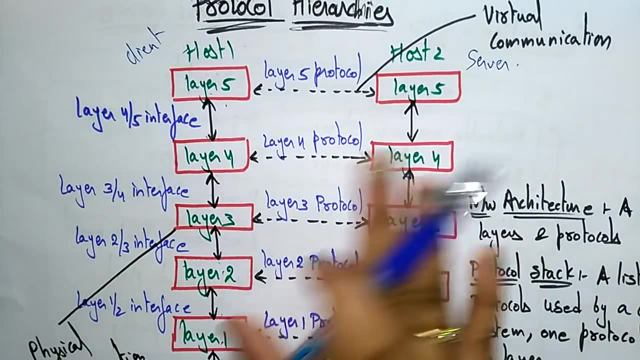 And here In between the layers, means in a single computer, in the host one or in the host two. within the layer you're having a physical communication. So this is a physical communication. within the layers you are having the physical communication, and outside the layers, between the two computers you have, they are having the virtual communication. 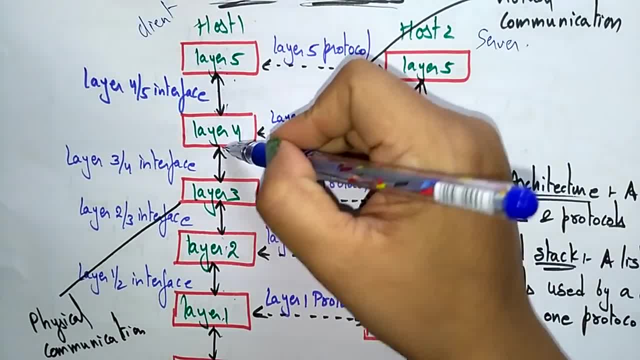 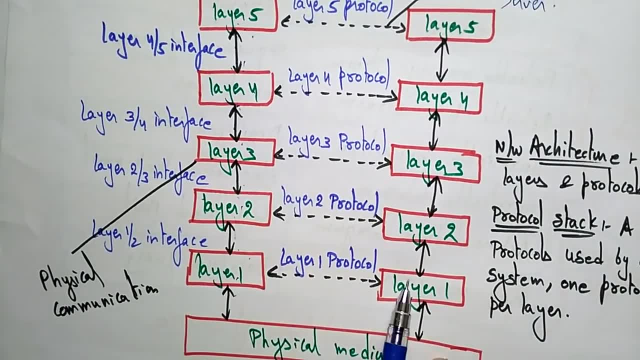 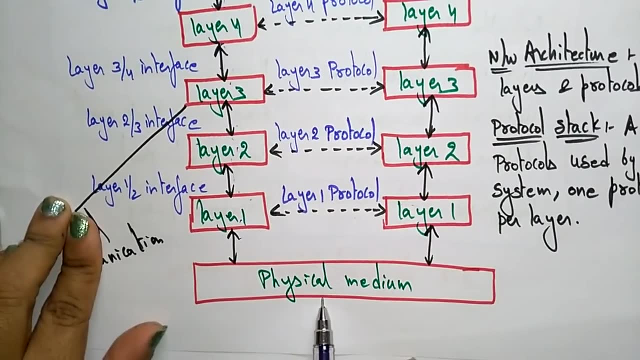 So this layer five is an interface of layer four by five and it acts as an interface of layer three by four and this is acting as interface two by three, three and one by two, and this is layer one, protocol, layer two, protocol three, four, five, and all these two- host one and host two- will be connected to physical media, the physical media. 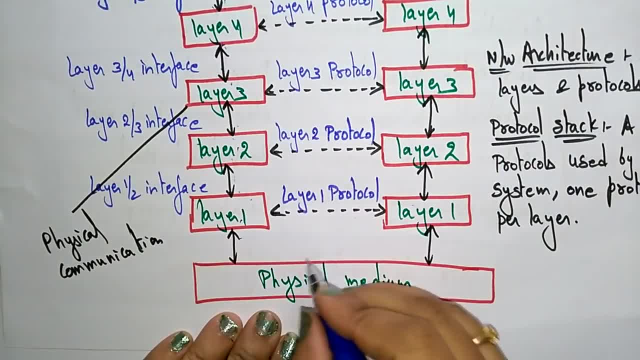 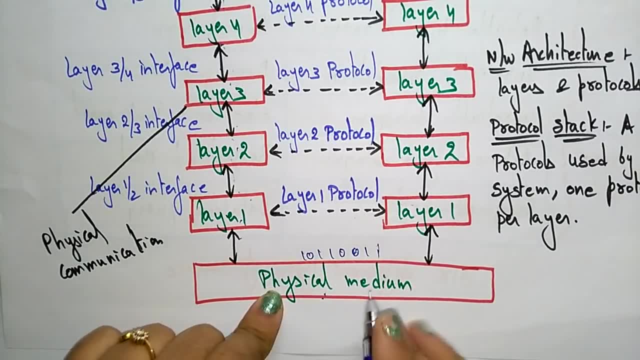 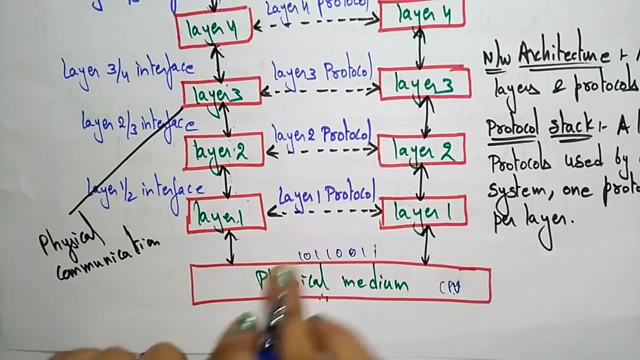 which is holding the converting all the data in the form of ones and zeros, so it accepts only the data in binary information. the binary information can be accepted and that which is accepted by the cpu. the cpu can accept only the binary data, so that will be converted in this physical media.